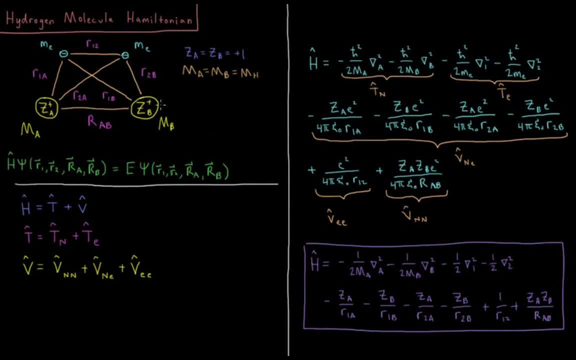 diatomic molecule are more apparent. But just anytime you see those for hydrogen, just substitute in the value one in your mind. The mass of each of those is equal to the mass of a hydrogen nucleus, which will be usually just one proton. We've got two electrons here. Each of them weigh, mass of the electron, have a charge of negative E. 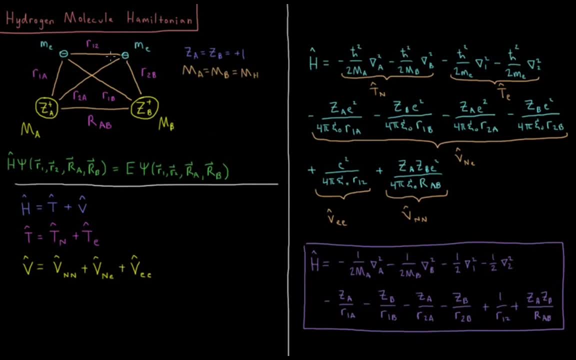 And so of these four particles, we have kinetic energy for each of them, which is of interest. But we're also interested in the Coulomb interactions between all six pairs of them. So six distances of note are from nucleus one- sorry, from nucleus A to electron one, R1A. Nucleus B to electron one. 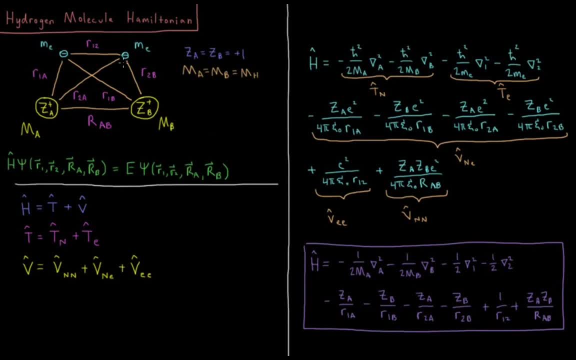 R1B. Nucleus A to electron two. R2A. Nucleus B to electron two. R2B. Electron one to electron two R12.. And what is new in this video and in this chapter is the distance between nucleus. 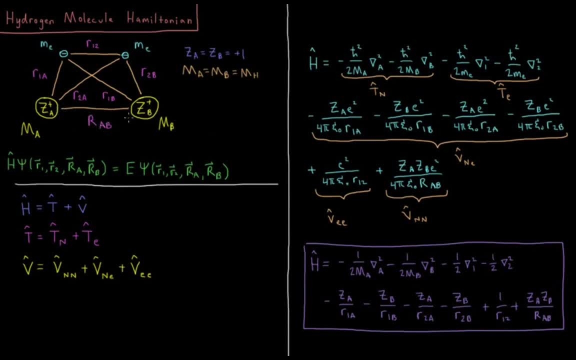 A and nucleus B, capital RAB. So in principle, our Hamiltonian and our wave function will be a function of 12 variables. They'll be a function of the three Cartesian coordinates of each of our four particles. So we have electron, one has three coordinates: Electron. 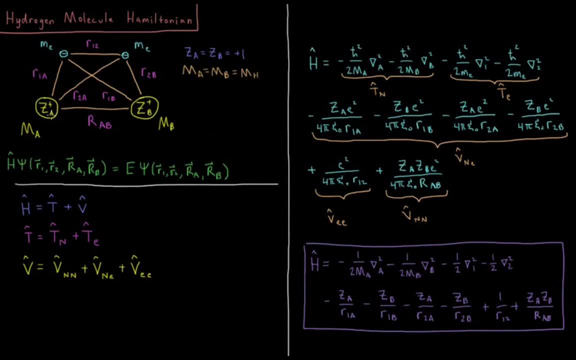 two has three coordinates. Nucleus one has three Cartesian coordinates, X, Y and Z, as does nucleus B. So our Schrodinger equation, H psi equals E psi, depends on us specifying our Hamiltonian operator to act on this 12-dimensional wave. 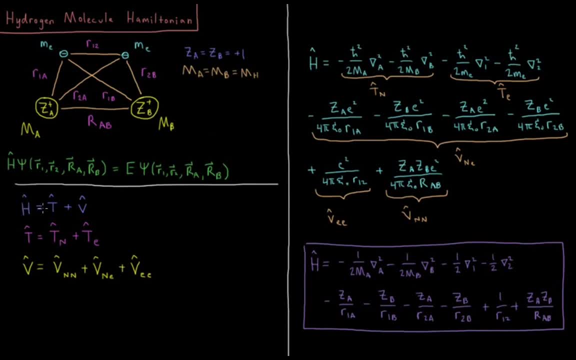 So our Hamiltonian, as always, is equal to the kinetic energy plus the potential energy. Kinetic energy is equal to the kinetic energy of the nuclei plus the kinetic energy of the electrons, And the potential energy is equal to the potential energy between pairs of nuclei. 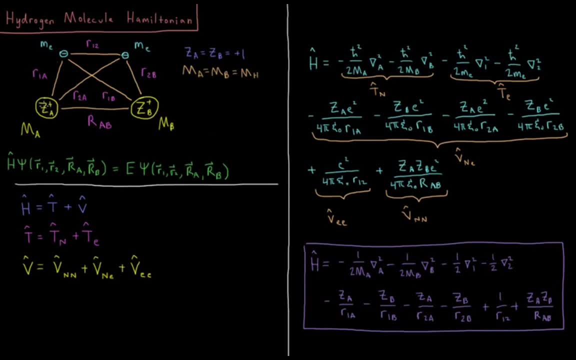 plus the potential energy between nuclei and electrons, all four cases of that plus the potential between pairs of electrons, electrons. so our total Hamiltonian writing that out, H, H hat is equal to kinetic energy of nucleus. a minus h. bar squared over 2. mass a del squared a. 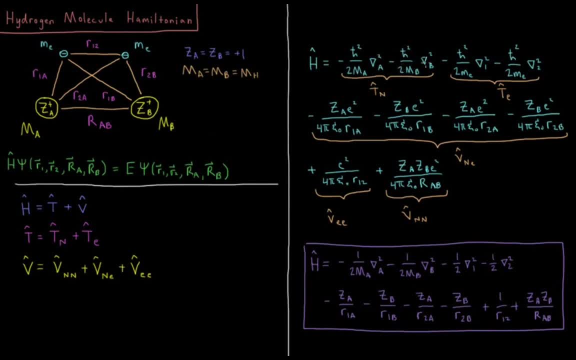 minus h bar, squared over 2 MB del squared B. second derivative: sum of the second derivative with respect to each coordinate in B. these each are: a nuclear kinetic energy term kinetic energy of our electrons minus h bar, squared over 2 times mass of the electron del squared 1 minus h bar, squared over 2 times mass. 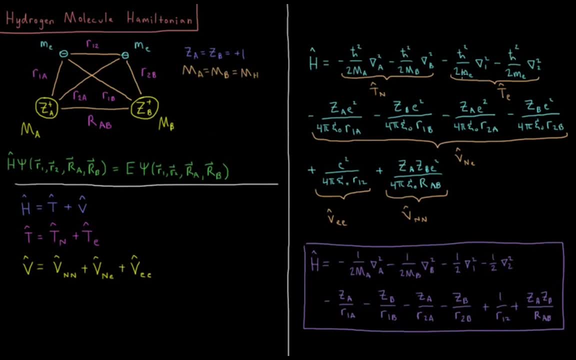 of the electron del squared of electron 2, those are the kinetic energy of our electrons terms. then we have four terms of electrons being attracted to nuclei, mine, and in each case the charge of the electron is negative e. charge of the nucleus is plus Z times e. so electrons and nuclei have opposite charges, so they will. 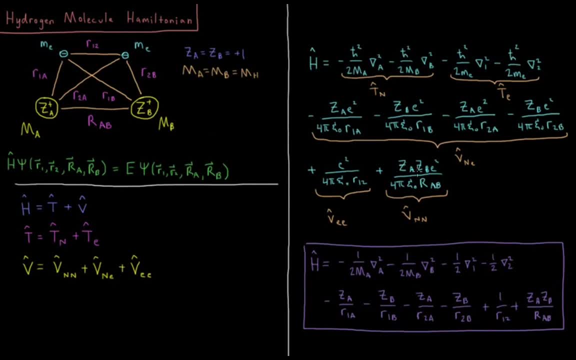 attract one another, giving a negative potential energy. so these terms are negative: Z a e squared over 4 pi. epsilon naught R 1 a minus Z. B e squared over 4 pi. epsilon naught R 1 B minus Z a. e squared over 4 pi. epsilon naught R 2 a. 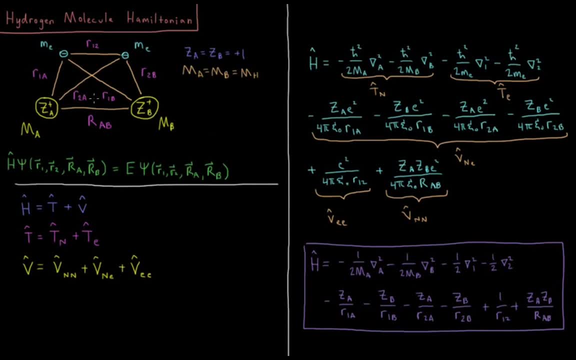 sorry, this was R 1 B. this is our 2 a and minus ZB e squared over 4 pi epsilon, not r 2 b. those are nuclear electron attraction terms. we have our electron electron repulsion terms, same sign: repulsive potential, energy positive potential, plus E squared over 4 pi epsilon. 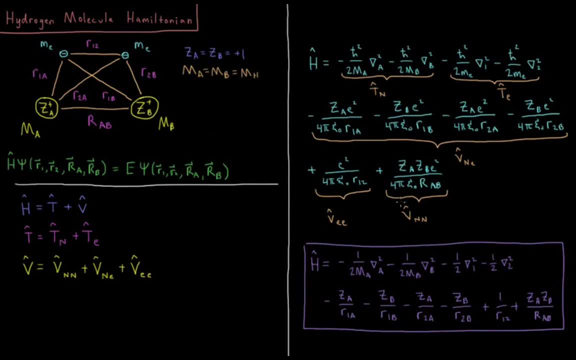 naught R12, and nuclear-nuclear repulsion terms: ZA times ZB. E squared over 4 pi. epsilon naught RAB. If we take all these terms and we put them into atomic units, where we divide, where we set a whole bunch of things to equal to 1, H bar is equal to 1,. mass of the electron: 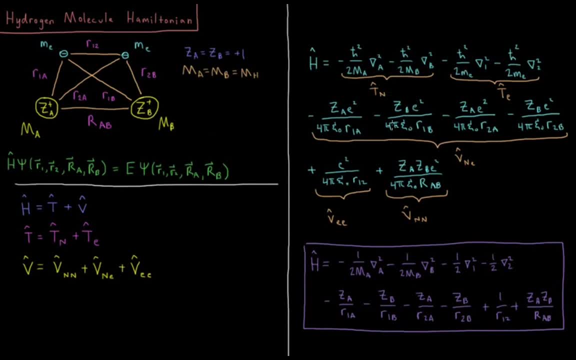 is equal to 1, charge of the electron is equal to 1, and 4 pi epsilon naught is equal to 1.. So what's left over is H equals minus 1 over 2 MA. this is now how many electrons worth.